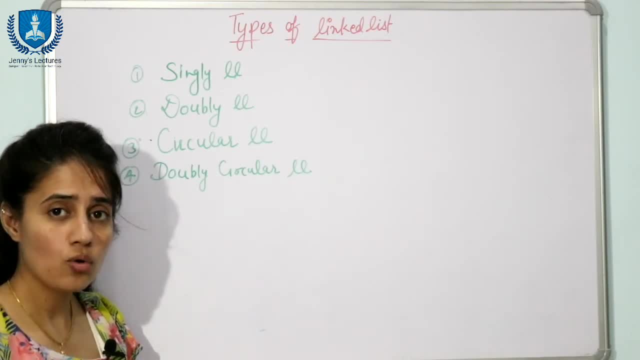 while implementation and you can implement your own type of link list. Fine. So first of all, we will discuss what is singly link list. Singly link list is the most common used link list. When you say link list, it means you are studying singly link list In singly link list. 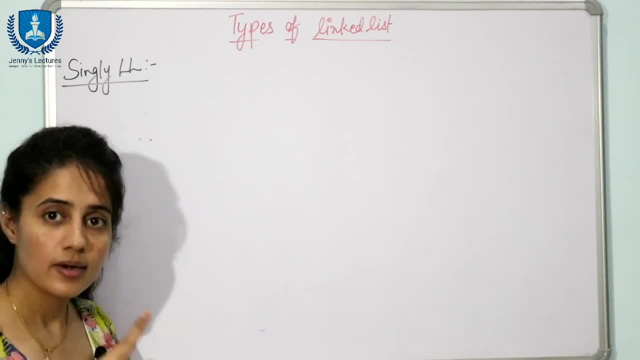 each node contains two parts. One is data part and next one is address part. Right, And that address part contains address of next node, or you can say address of the successor node, Fine. Or you can say: in singly link list, each node contains data part and a pointer to its next node. 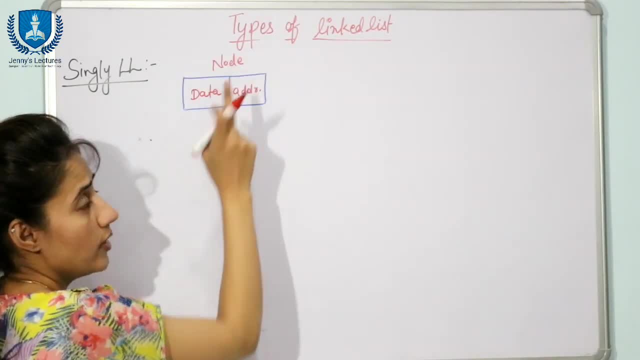 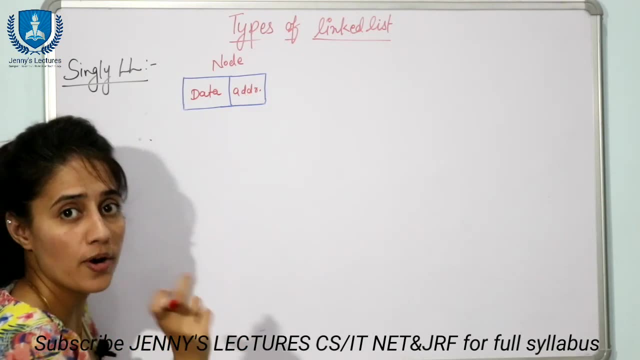 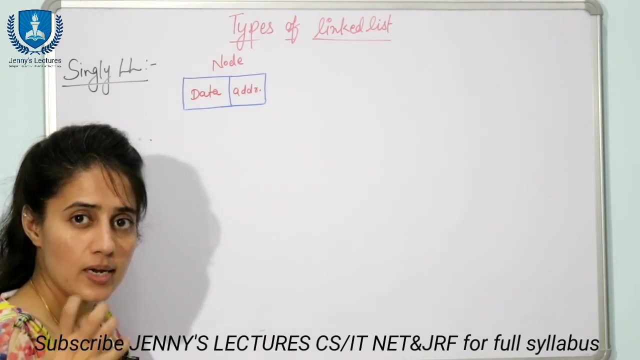 Right, See, like this. See, this is a node in the singly link list. It is having two parts. This is data part and this one is address part. Or you can say this is pointer Right, Pointer to its next node. Right Now. if suppose a singly link list contains three nodes, then how you will represent? 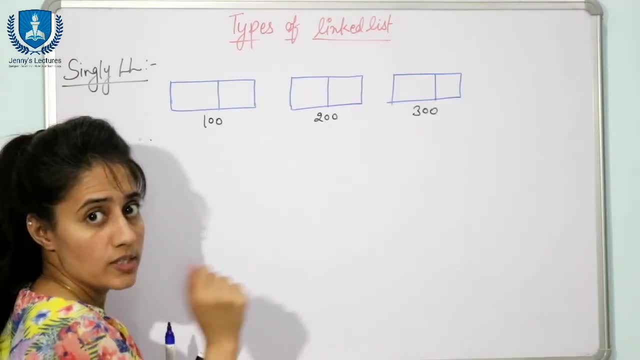 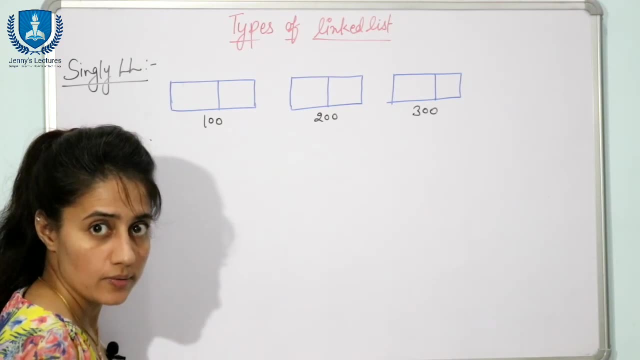 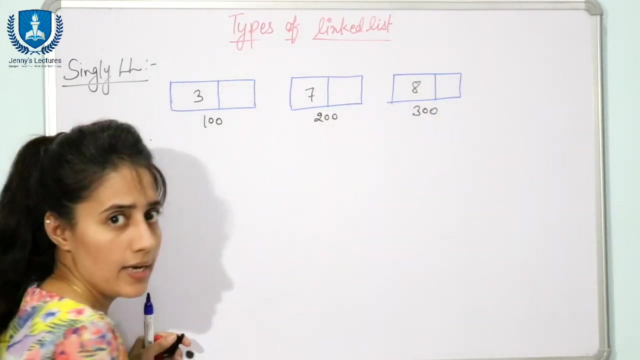 that list See. So these are three nodes. Each node is having its own address in the memory: 100, 200 and 300.. And this node, the data part of this node, is suppose it contains three, it contains seven and it is having eight. This is what the address part. or you can say a pointer or you can. 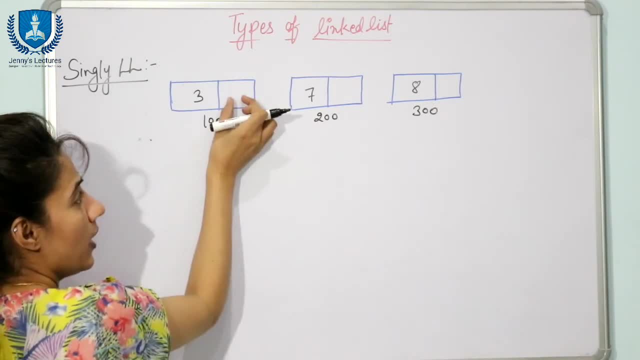 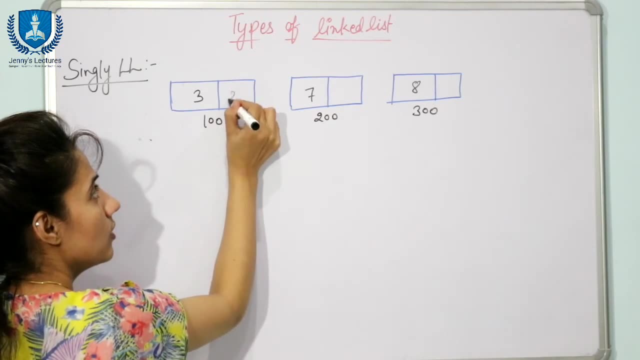 say a link, Link to its next node. So this part contains address of the next node. Suppose this is the next node. Address is 200. So here you will write what: 200. So it is going to point to. 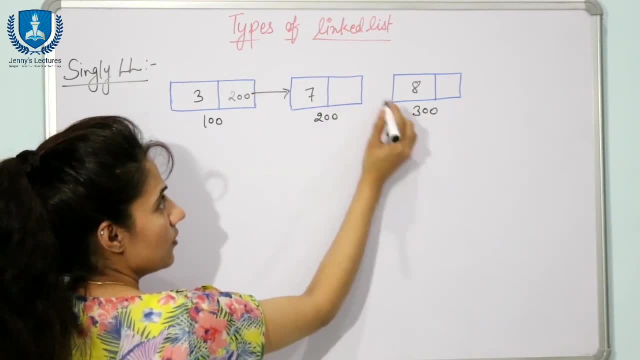 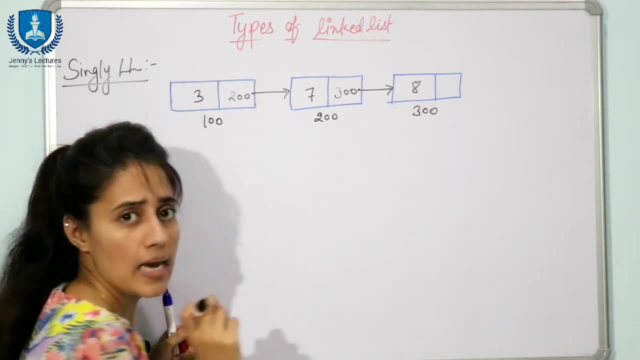 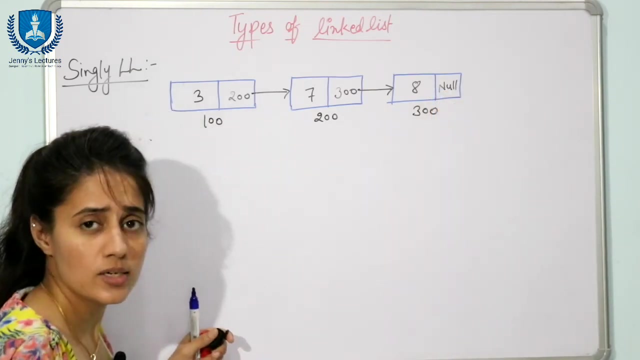 this node. This contains what Address of next node? that is 300. So it is going to point to the next node And suppose this is the last node. So the address part of last node contains what? Null, You can say zero, It is not going to point anywhere. And the address of this first node is: 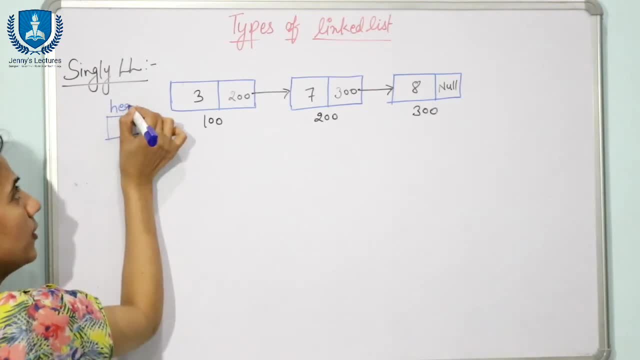 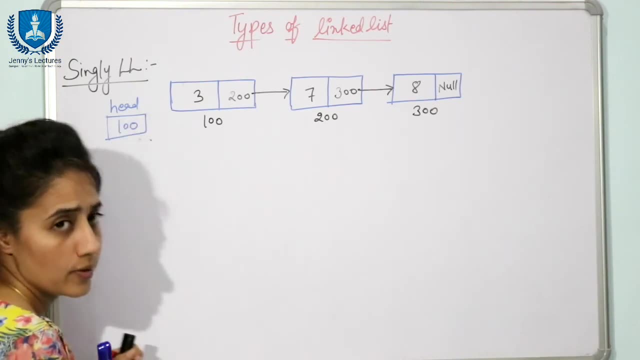 stored in a pointer- You can say head pointer- or a start pointer- In which this address is going to be stored, Right. So now this is going to point here. See, this is not a head node, It is a pointer only Because it is going to store only the address of 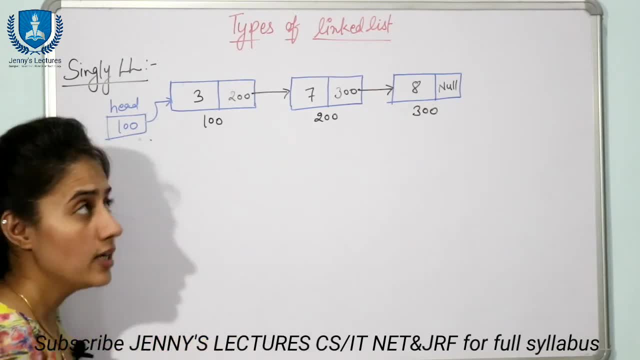 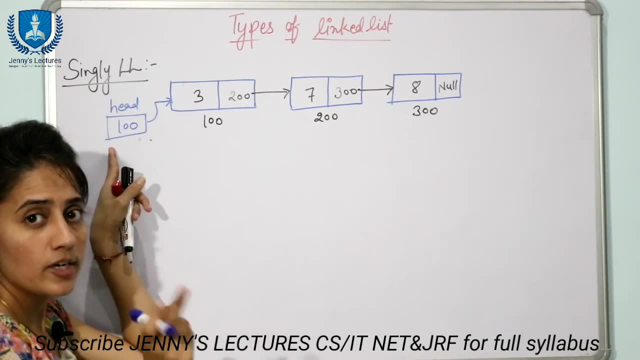 this node. If someone is saying head node, it means this is the head node. It is not the node, It is just a head pointer or start pointer. So when you are going to write a program, then you are going to maintain only this head pointer. 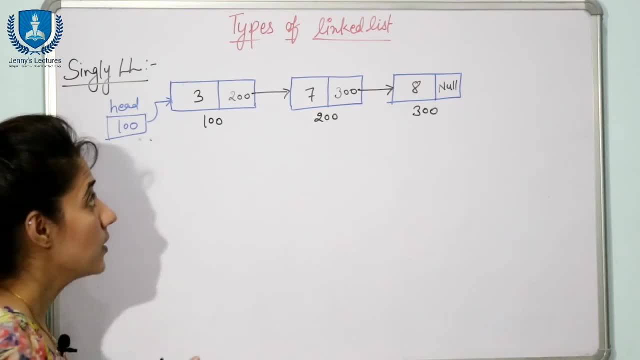 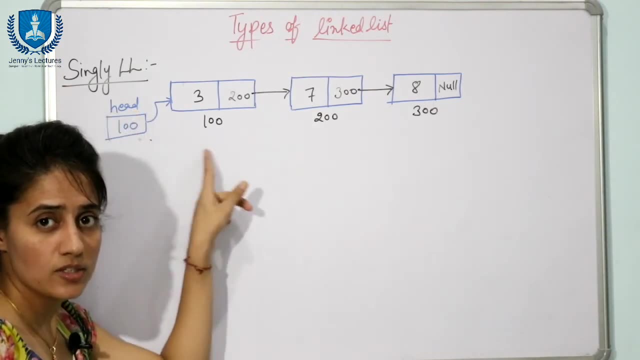 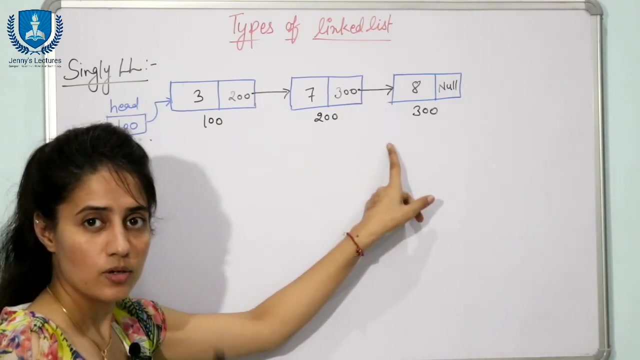 See address of the node. First node: Fine, See, this is what a singly linked list. See why this is known as a singly linked list. As the name suggests, this is having only a single link. See, this is a single link, only Single link to its next node. So here in this list only. 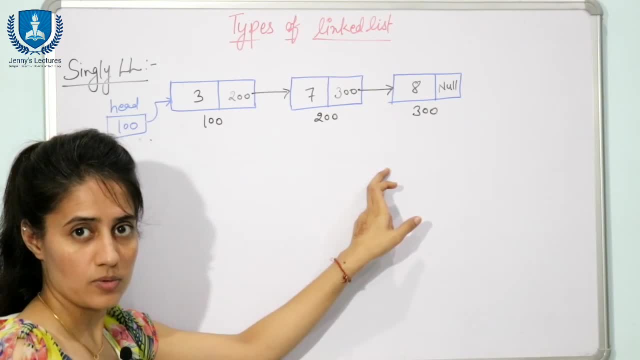 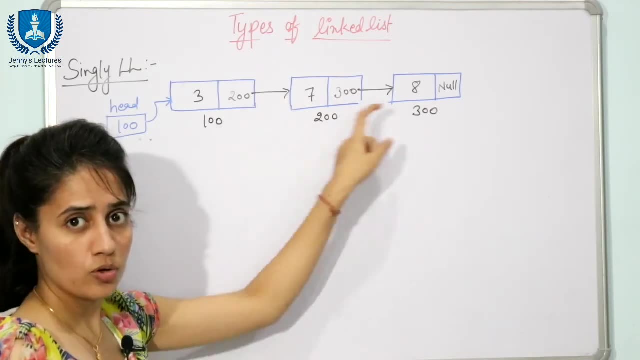 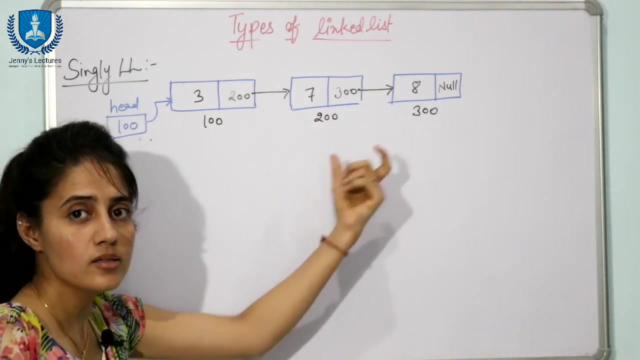 forward traversal is possible in the list. You cannot traverse the list in backward direction Because this is having only one direction That is going to be forward. Or you can say: in this case only forward, sequential movement is possible. Now how we are going to represent this node when you are going to write. 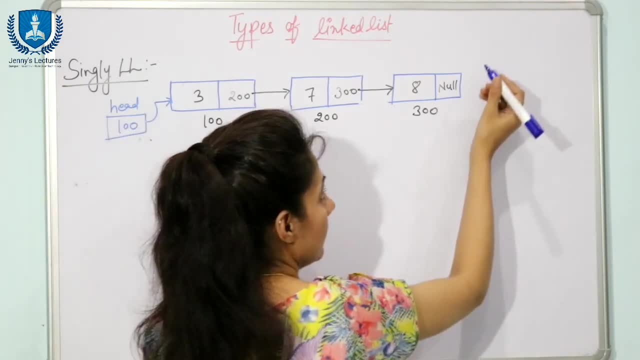 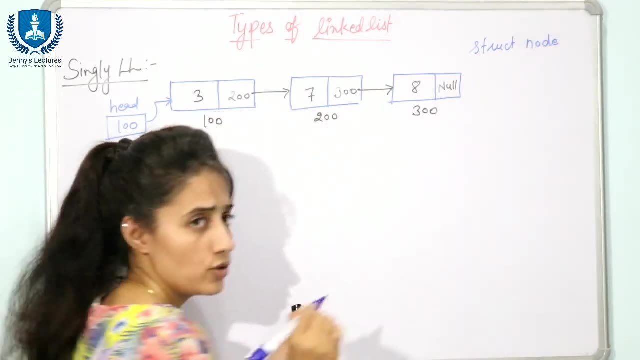 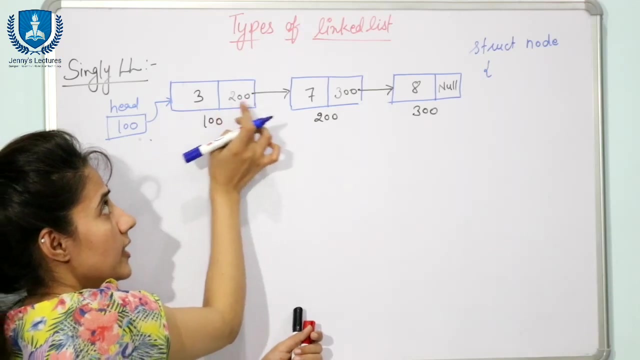 a program That we have already discussed. I am going to write here. See how we are going to represent that. We are going to write struct node, A user defined data type. that is structure, Fine. And in this node we are having two parts: Data and address. So you can say int data, You can say any variable. 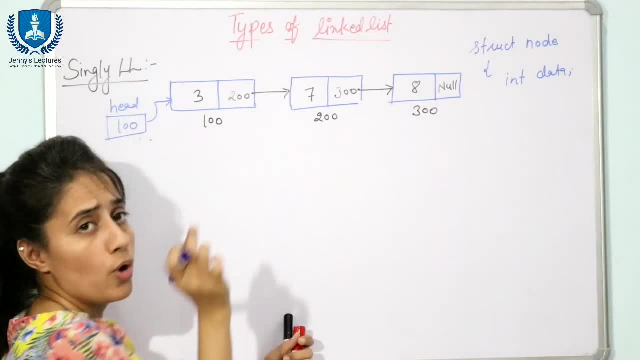 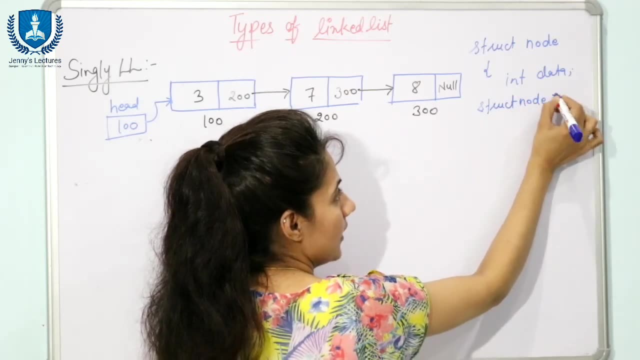 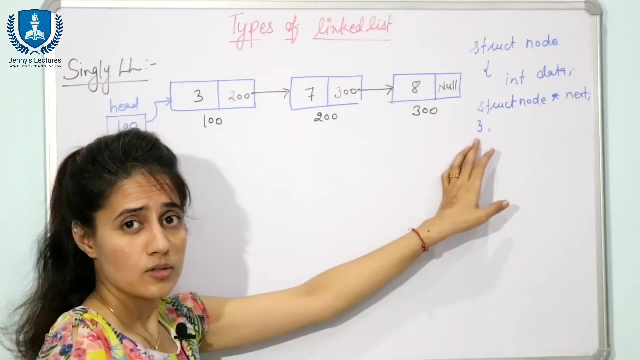 a or x or something like this. Fine, Next is pointer Pointer to next node. So here you will write what Struct node, asterisk, and the name of pointer. you can say next or link, as you wish. So this is the representation of the node Right In the program. 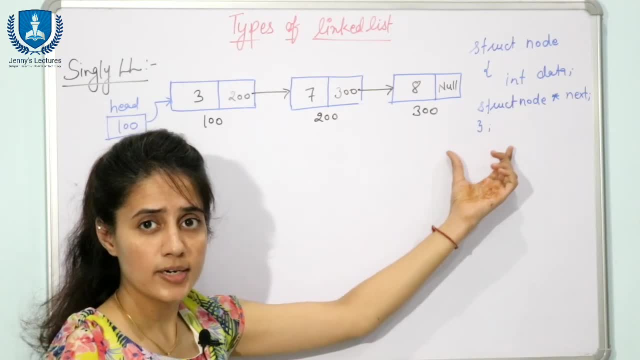 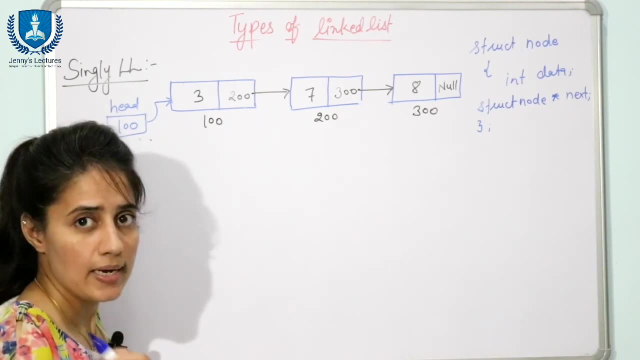 Why am I writing here? struct node that I already discussed in the previous video. You can check out There. Fine, See now. Next is doubly linked list, As the names suggest, see doubly linked list. It is going to have. 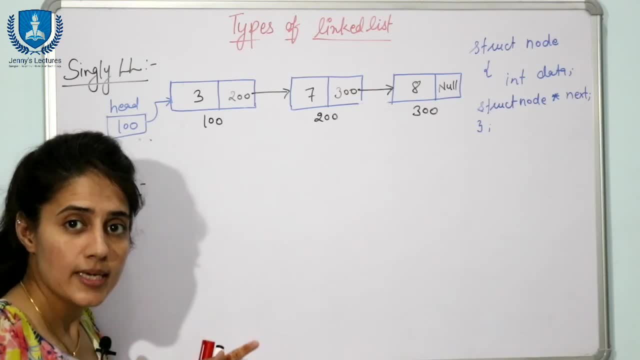 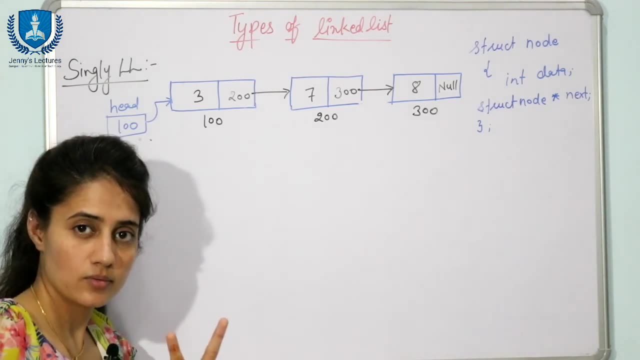 double pointer, Two pointers, Fine, So in this case each node is having three parts. One is data part and two address part. Right? Or you can say each node is Right, Or you can say each node is having. 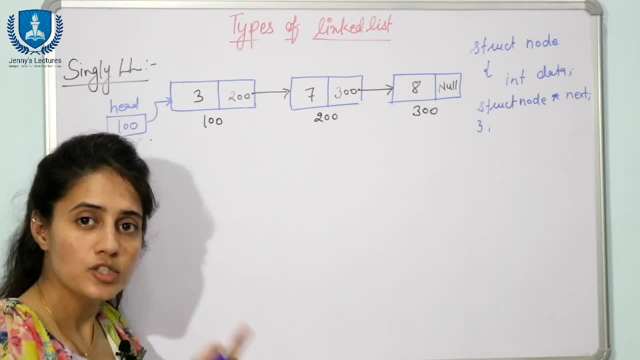 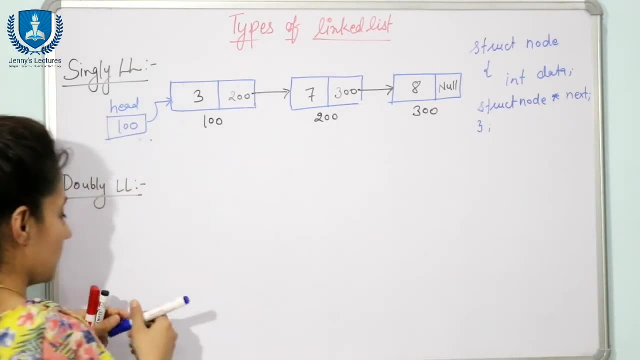 Right. Or you can say each node is having Right, Or you can say each node is having data part and pointer to its previous node and pointer to its next node. two pointers would be there. right, something like this: three parts would be there. this is a node. this is node in double. 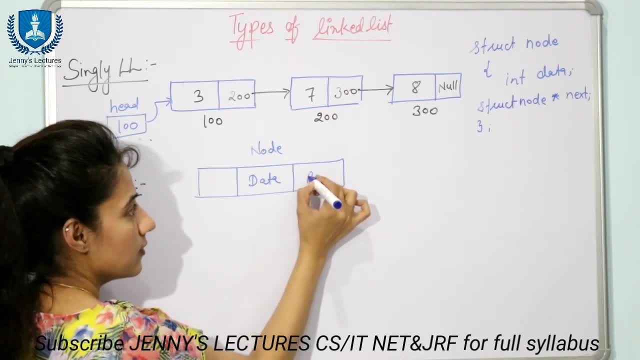 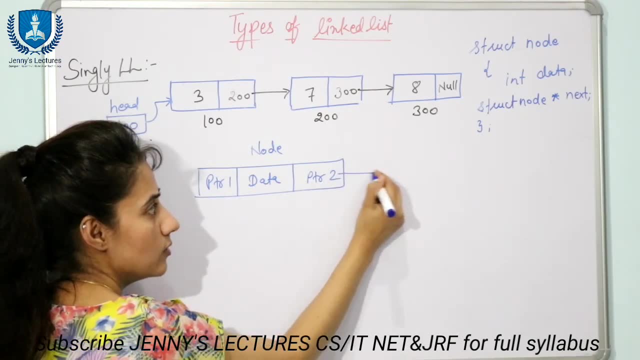 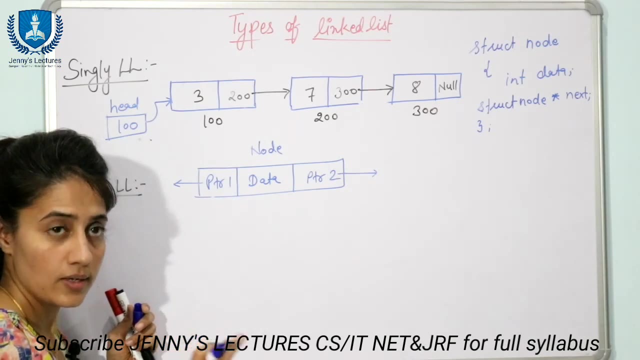 linked list it is. it is having three parts: data part. this one is you can say, you can say pointer one and pointer two. so this pointer is going to point the next node in the list and this pointer is going to point to the previous node in the list. right, in this case we are having only single. 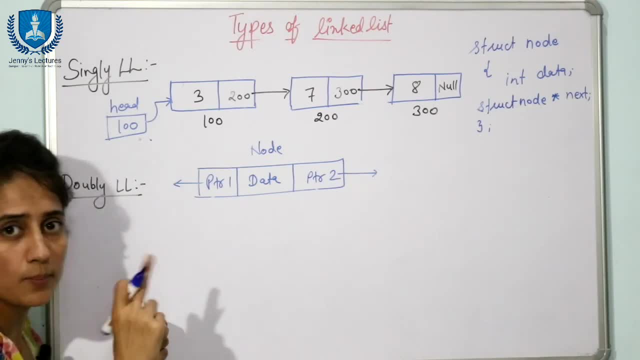 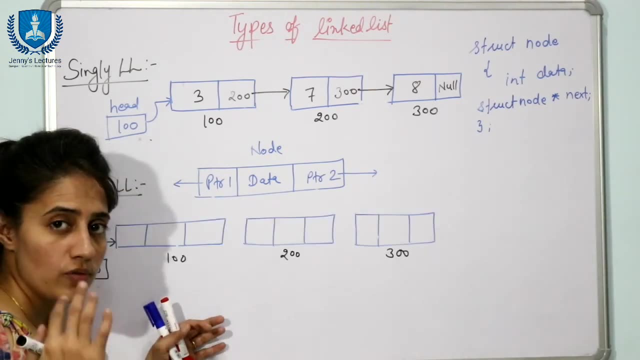 pointer. in this case we are having two pointers. that is why we are going to call it double linked list. right, so now how to represent this double linked list? see. so suppose in this case also we are having three node. in the double linked list, see, three parts would be there and the data part. 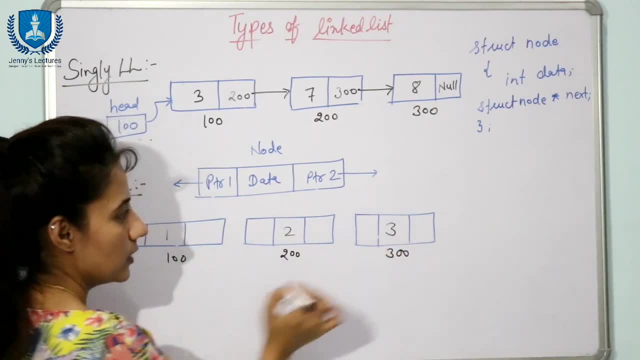 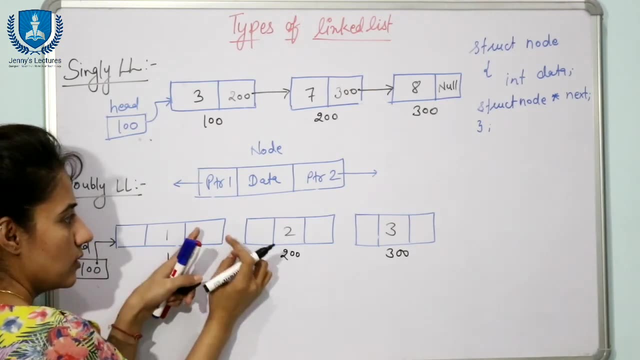 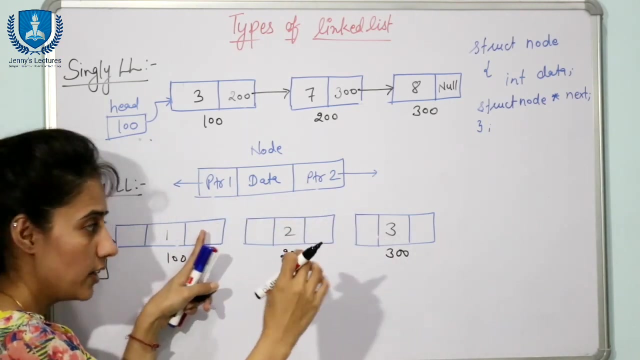 suppose contains one, two and three, three integer values now. so if we drop the side, it is going to say that this is only one node and this is only one point. this part, this pointer, contains the address of next node in the list. fine, in the sequence of elements, right. so the next node is this one address is 200. so 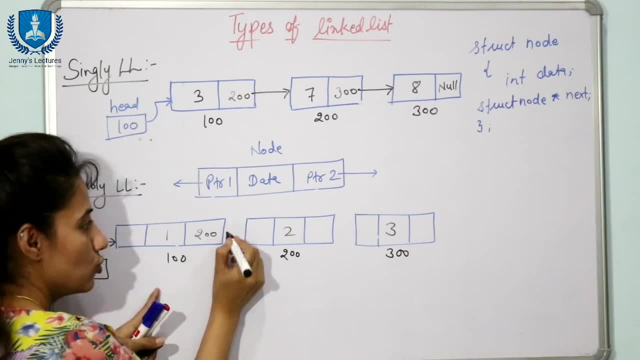 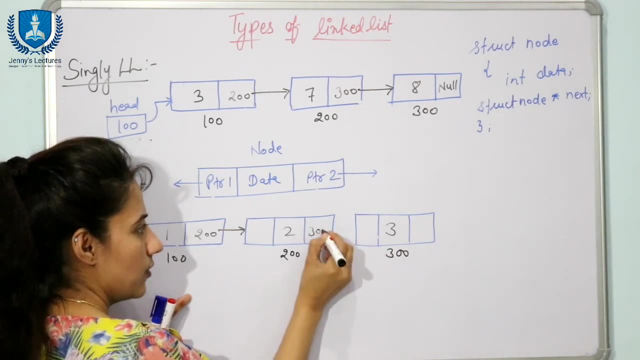 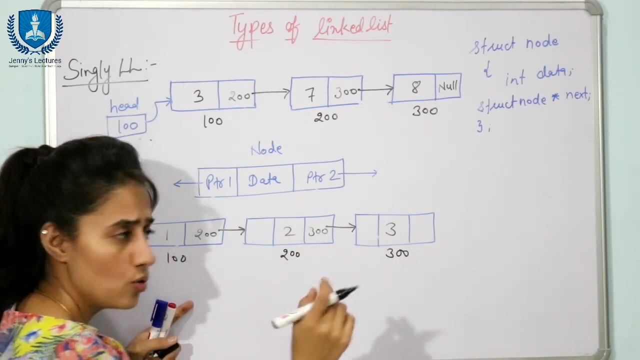 this node can? this part contains 200, right, so this is going to point here now. in this also, we are having 300, the address of its next node, so it is going to point here. fine, and suppose this is the last node. so in this and in this, 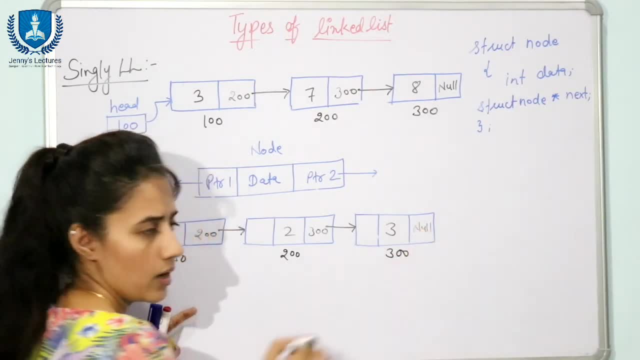 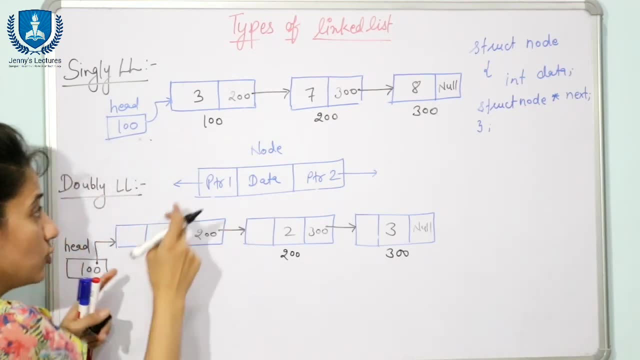 part, the pointer 2, it is going to have null, or you can say a 0 because it is not going to point anywhere, right? so now? second pointer is pointer 1. this node is having this. the sorry, this address part is having address of its previous node. 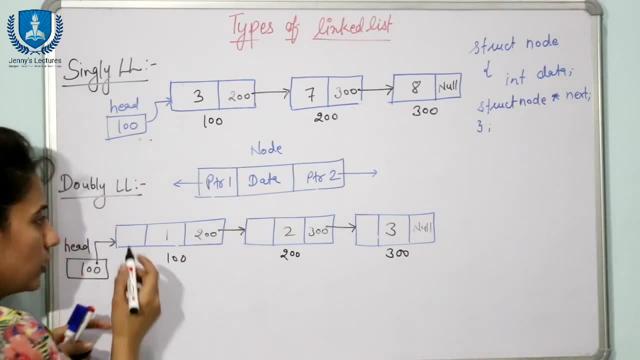 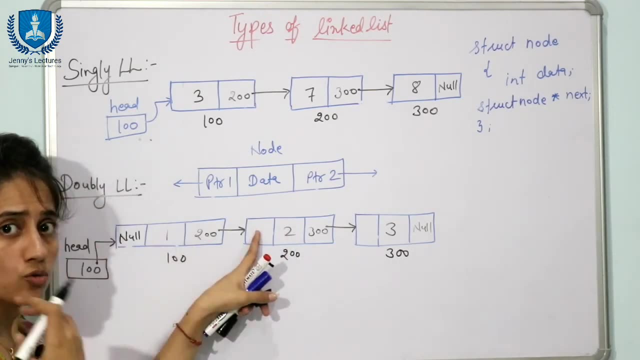 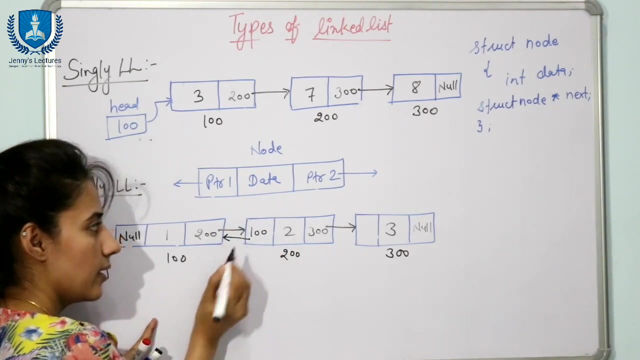 but this is the first node. no previous node is there. so it is going to have null and this part of this node is having address of its previous node. previous node is this one address is hundred, so it is going to have hundred. so it is going to point here. right now. the link is from here to here. this is having. 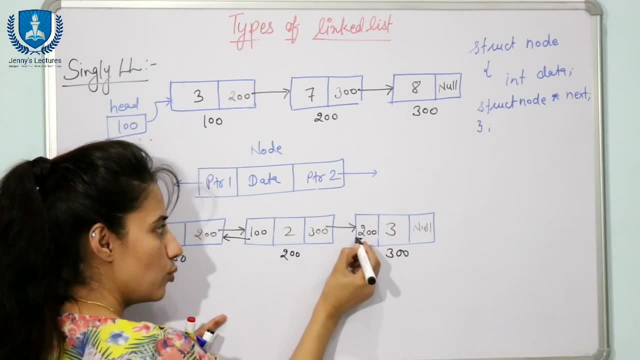 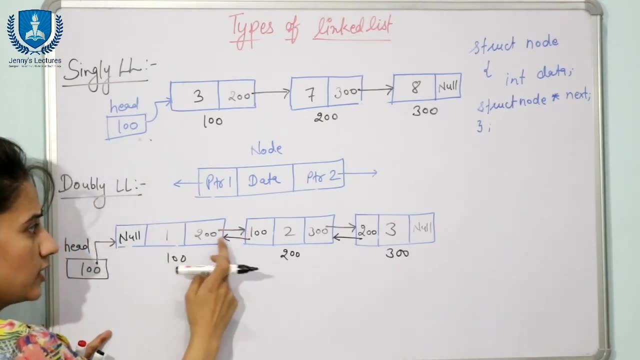 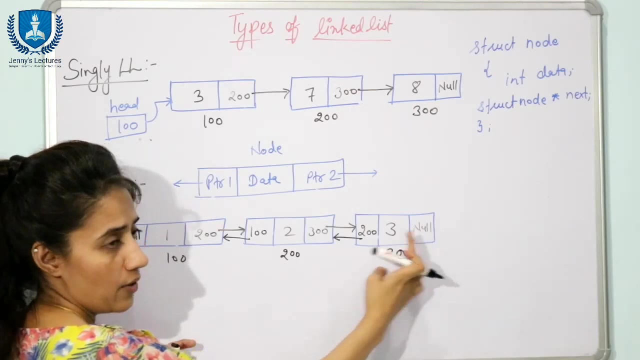 address, 200, address of its previous node. so it is going to point here. fine, so double links are there? two links are there. one is in forward direction, one is backward direction and in the last node there is no successor, no next node. that is why this pointer is having null and in the case of first node there is no previous node. 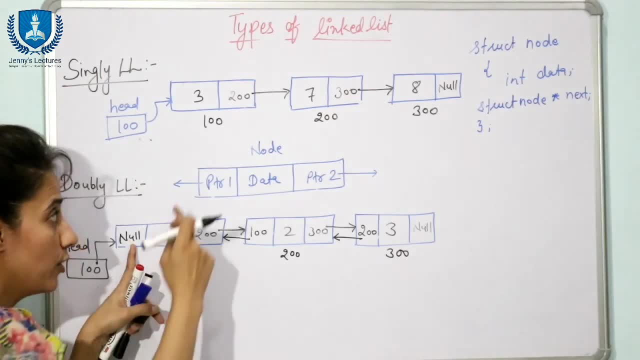 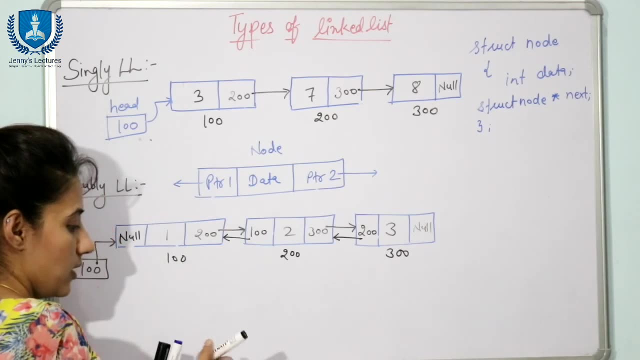 so this pointer is having now the first, the pointer one now, how we are going to represent the node of a doubly linked list when you are going to write a program, see same types. data type would be there. we are going to define a strap- nové's Ones. 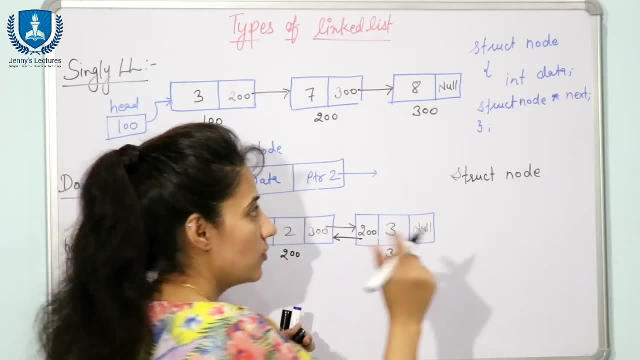 or trough node is a data type, name of data type. this is user defined in our uh theme. if you want to be own user, need some data type. if you want to be run by, is user defined in a type right within this node. we are having three parts now, so one is integer. 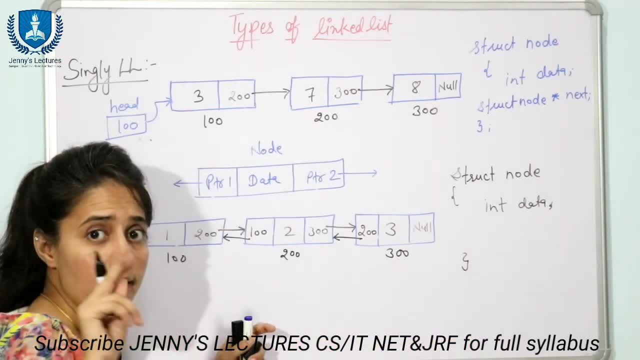 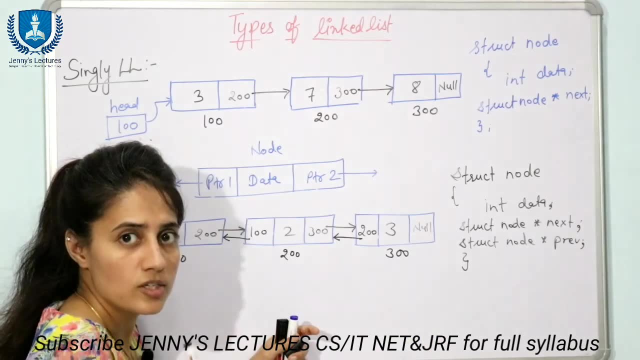 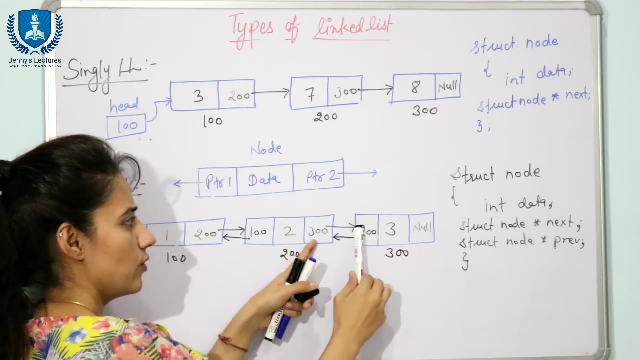 you can say data part, right, and two pointers. so the type is what struct, node only. so this is how we are going to represent it. two pointers would be there. one is next. this one is next means you are going to store the address of next node and previous. this is previous. this is going to store. 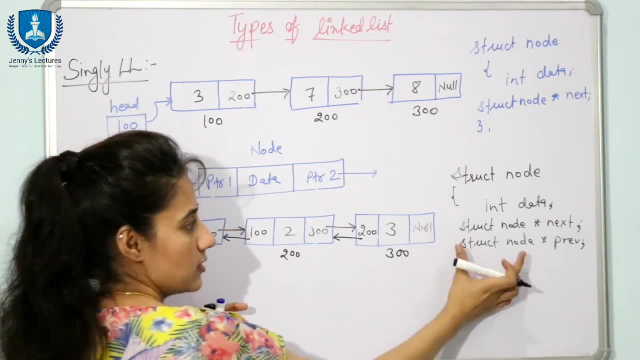 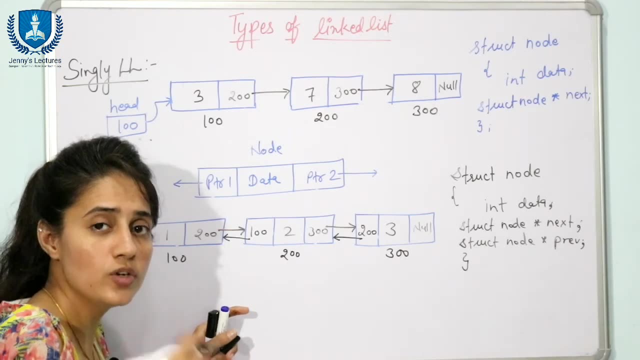 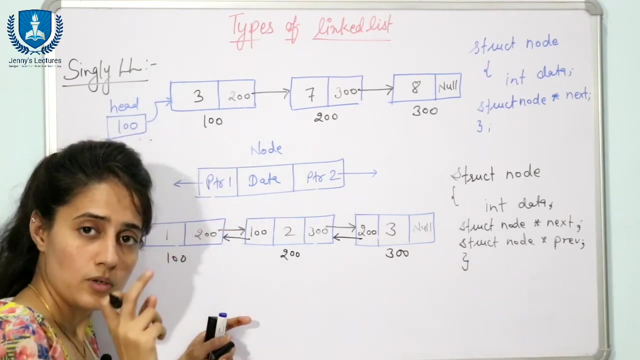 address of previous node. right why this type is a struct node? because it the pointer. this pointer is going to store address of which type of node. type of node is struct node. and here i always will write what the address of the elements whose address the pointer variable is going to store. 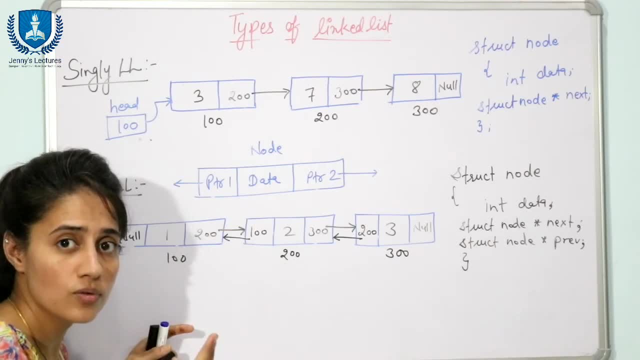 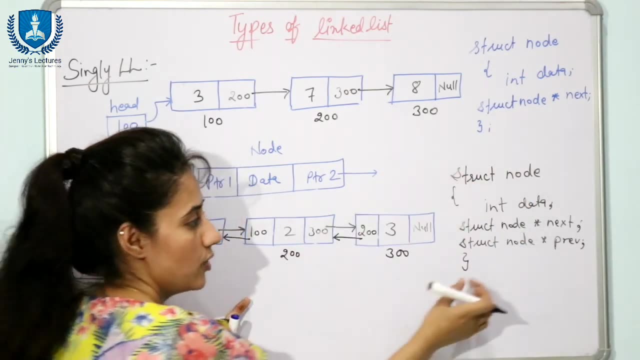 right. so here pointer variable is going to store address of, not a simple variable, address of a particular node, and the type of this node is what: struct node. that is why we are writing here: struct node. this is how we are going to represent this node when you are writing a program for a 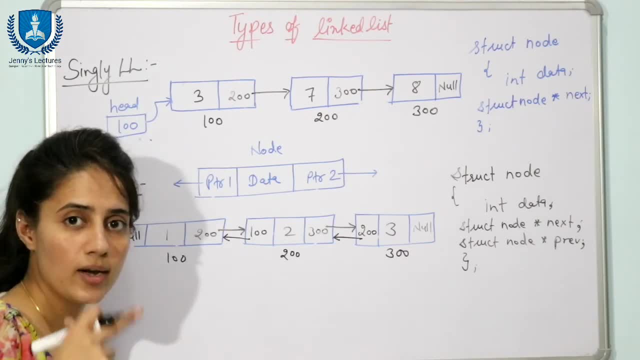 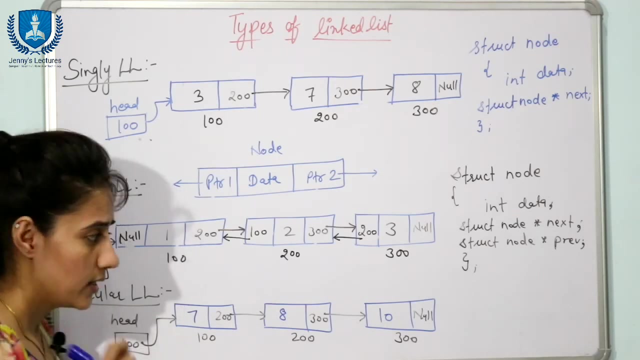 doubly linked list right now. third one is circular linked list, see circular linked list. as the name suggests, it is going to have a circle. so circular linked list is a variation of singly linked list, or you can say it is a singly linked list. the only difference is what see in. 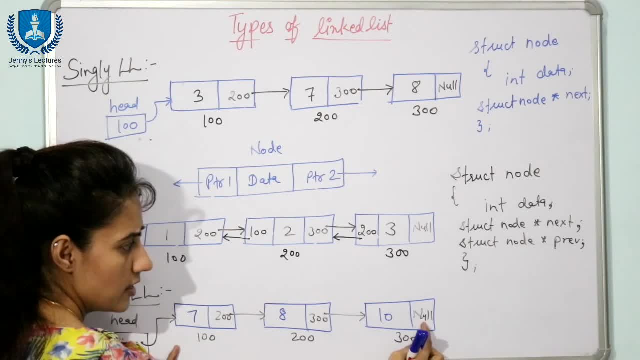 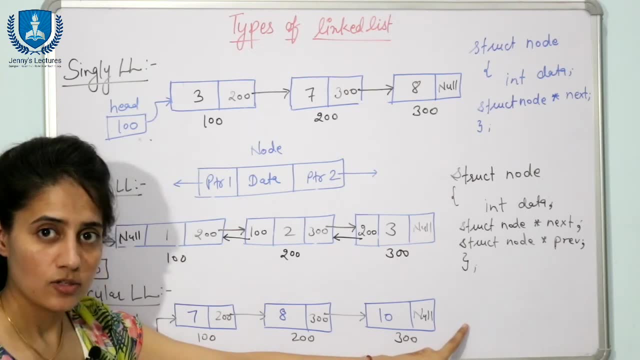 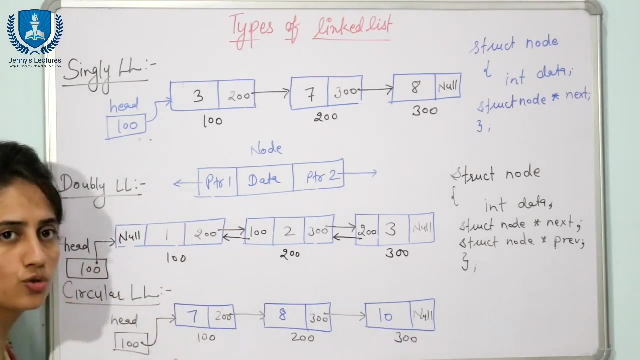 this is singly linked list. in singly linked list, this last node is having what null? it is not going to point anywhere, but to make it a circular linked list, what you are going to do in the last node of this list we are going to store address of first node, right. so now address of first node. 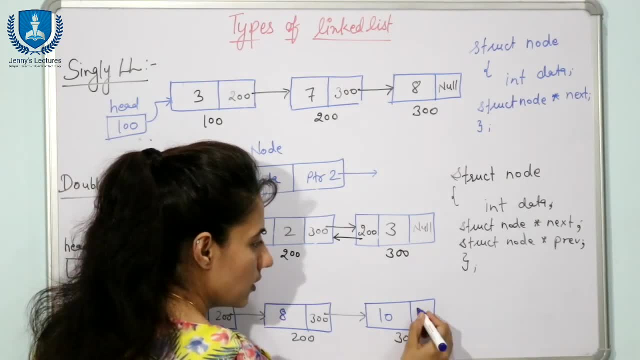 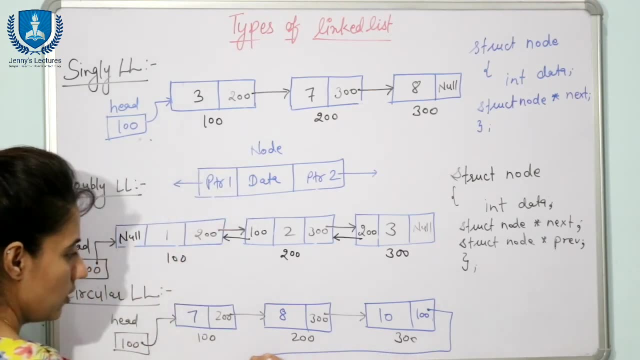 is what hundred. so here you are going to store hundred. now this node is going to point where, to the first node. so it is now a circular linked list. you can see, so you can say a circular linked list is a sequence of elements in which each element is having a link to its next element. 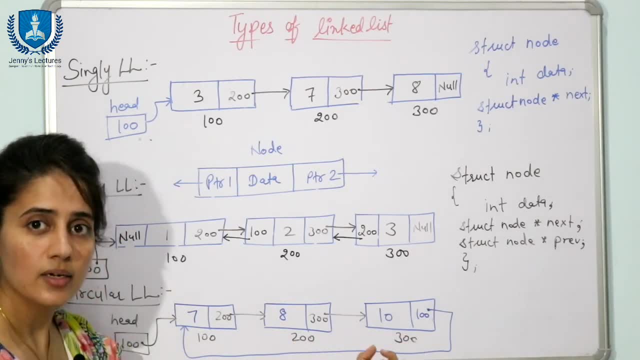 and the last node or the last element is having link to the first element in the list, right, so this is circular linked list. now, last is what doubly circular linked list. when i say circular linked list, it means it is what singly circular linked list. next variation is: 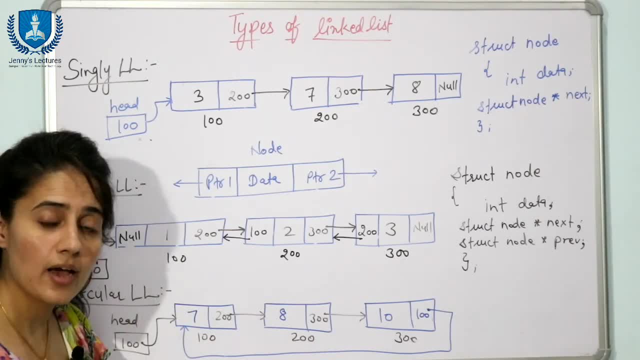 what doubly circular linked list, so that list is having properties of both doubly linked list as well as circular linked list. fine, so how we are going to represent that thing, see in this case, node is what node is having only two parts: data and address part. so in the 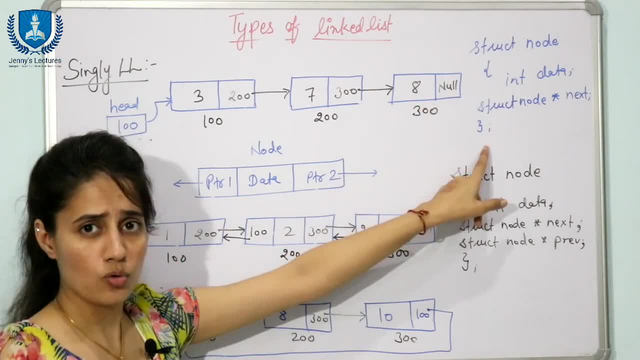 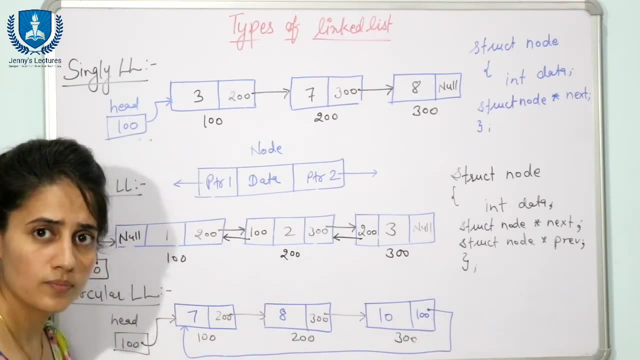 uh, that program. you are going to represent the node like this. only only difference is you are going to state one part intentions, something else ok, but when you say this additional, just like Mister walks towards the next one, and then just like Mister steps towards the next one, and same I. 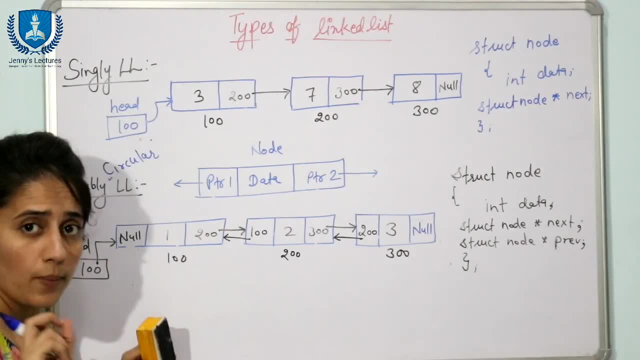 can just say you going to say locker ones or they belong to the first node, Fine, so in the buttons 아델 and the remote part, i said we are going to store a little bit in the last node. you are going to store address of first node. fine, and address of first node is.